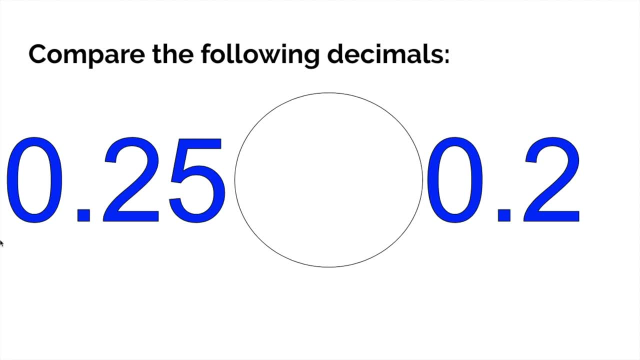 situation, all you want to do is take it place by place. For example, the ones place, they both have a zero, So they're still the same. The tenths place, they both have a two from the tenths place. Okay, still the same. Now here we have a five in the hundredths place and we have nothing in the 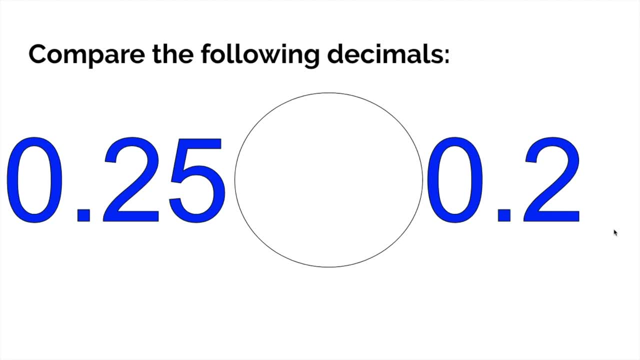 hundredths place in this number, And you know what? Nothing reminds me of zero. I know that five hundredths is greater than zero hundredths, So I'm thinking twenty-five hundredths must be greater than two tenths. And just for the fun of it, since we know there's nothing here, let's go ahead and 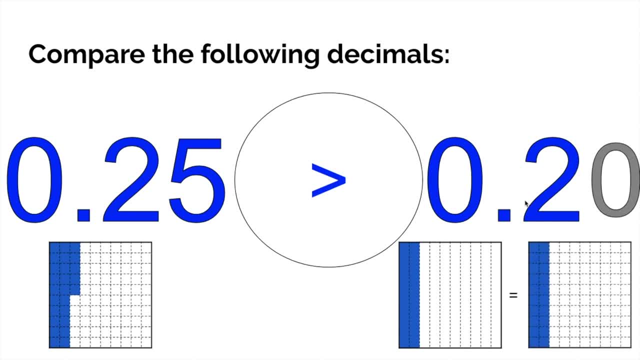 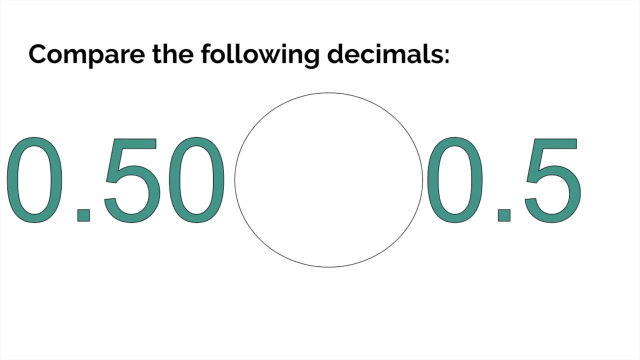 put a zero there and pretend it's twenty hundredths. Now it's easy to compare: Twenty-five hundredths is greater than twenty hundredths, which is two tenths. Two tenths is the same thing as twenty hundredths. Let's do it again Now, before you jump into it, talking about fifties bigger than five, let's do it one place at a time. 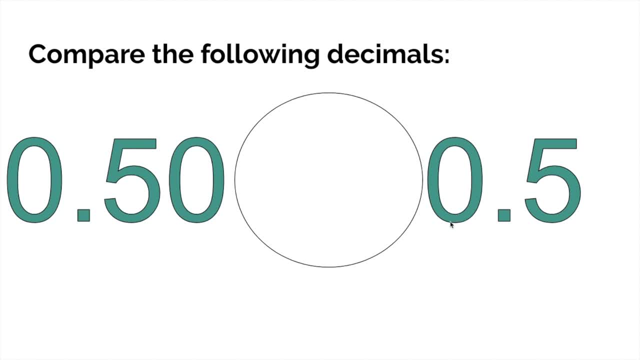 Okay, so ones place zero, zero, They're the same. Tenths place five, five. They both have five tenths. Let's keep it moving. Hundreds place zero, nothing which is zero, They're the same. 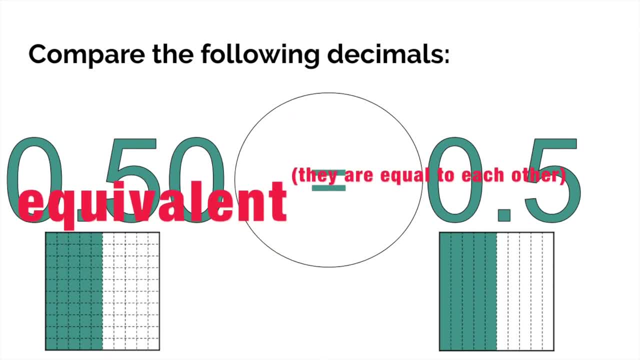 These are what we call equivalents. Alright, Fifty hundredths, five tenths- the exact same thing. Uh-huh, See, some of y'all was about to jump into it. It's like: oh yeah, fifties bigger than five. No, you need to stop it. 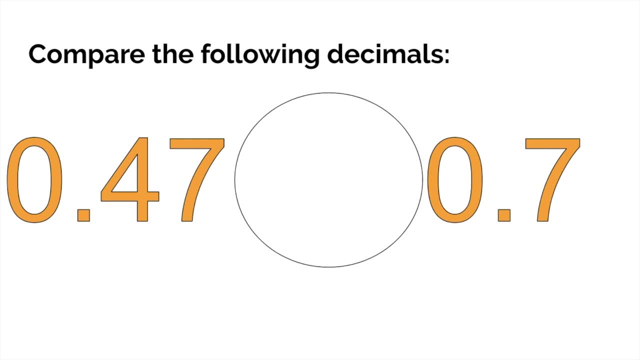 Take it one step at a time. Let's try this one again. One step at a time, Ones place. they both got zero Tenths. place four tenths, seven tenths. We're done. Seven tenths is bigger than four tenths, which means 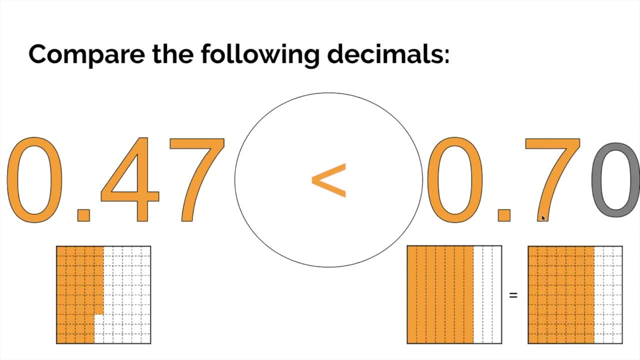 seven hundredths is less than seven tenths. If it helps, you can say: oh, there's nothing here in the hundreds place, so that's zero hundredths. So that's seventy hundredths is bigger than forty seven hundredths. Now you're like: oh, oh, yeah, yeah, yeah, you're right. 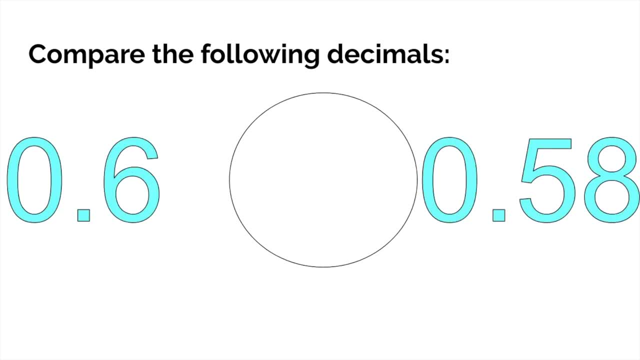 Seventy's bigger than forty seven? Uh-huh, That's what I thought. One step at a time. Do it one step at a time, Matter of fact. pause the video and do this on your own. Which one's bigger? Welcome back. I am assuming you paused the video.